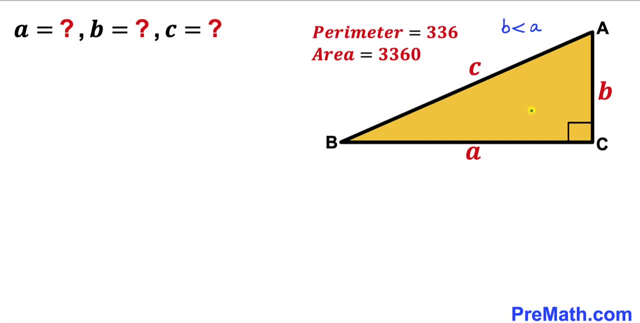 Welcome to PreMath. In this video we have got this right triangle ABC, as you can see in this diagram, such that its hypotenuse is represented by lowercase c. Its base side is represented by lowercase a And this side, AC, is represented by lowercase b. And keep in mind that side length b is less than a And furthermore, the 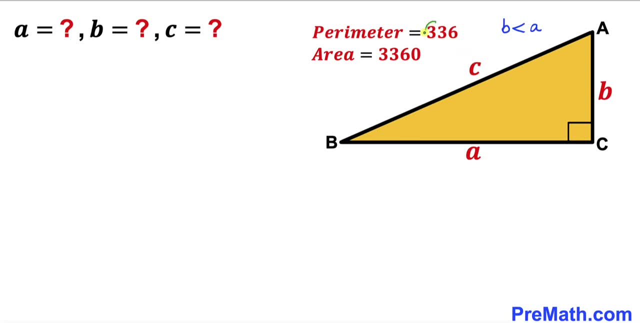 perimeter of this right triangle is 336 units, whereas its area is 3360 square units. And now our task is to find the value of these side lengths: a, b and c. Please don't forget to give a thumbs up and subscribe. Please keep in mind that this figure may not be 100% true to the scale. Let's go ahead. 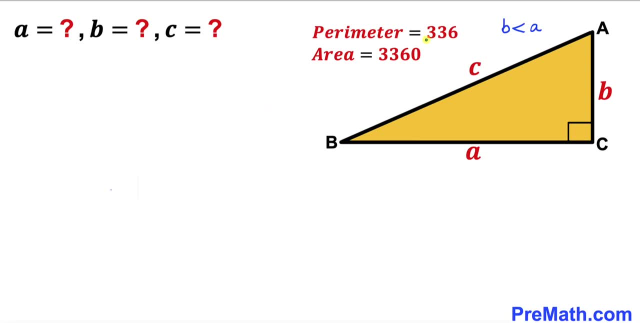 and get started, And here's our very first step. We know the perimeter of this given right triangle is 336.. And we know that the perimeter are just simply the sum of these three side lengths of the triangle, as you can see in this equation. And now we are going to replace this perimeter by. 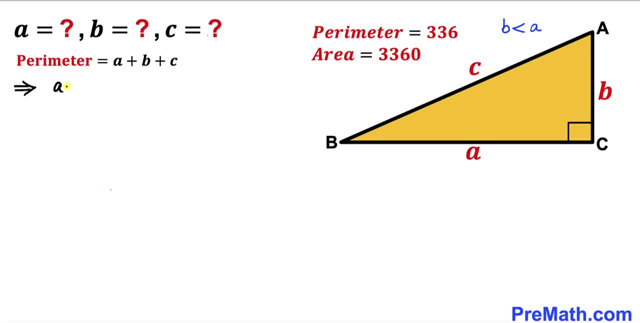 336 over here. So therefore we can write: a plus b plus c equals to 336.. Let me go ahead and call this as our equation number one, And here's our next step, since we are dealing with this right triangle. So therefore, let's recall the Pythagorean. 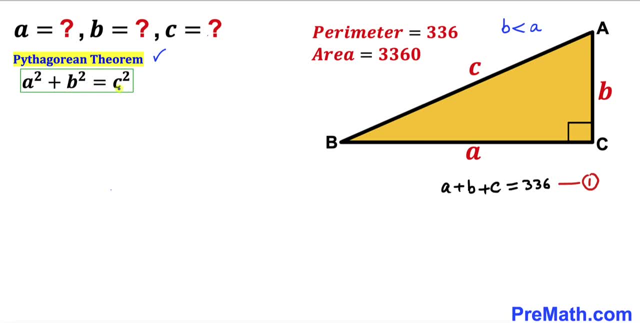 theorem: a square plus b square equal to c square. Let me call this our equation number two. And now let's recall the area of a triangle. formula Area equals to a half Times the base times height, And in our case our base is represented by lowercase a And height is: 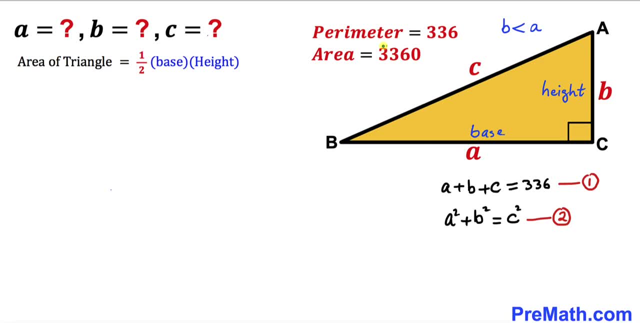 represented by lowercase p And the area is 3360.. So let's go ahead and fill in the blanks. this one in this formula: So this is 3360 equals to 1 over 2 times a, b. And now let's go ahead and multiply. 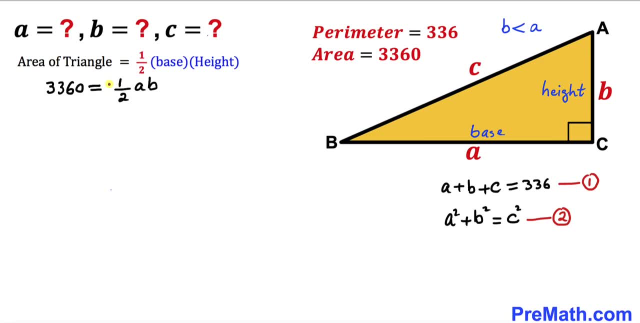 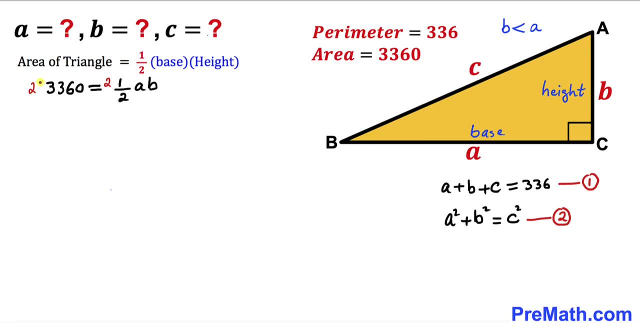 So I'm going to multiply this side by 2.. And over here on the left hand side by 2 as well, And now we can see 1 over 2 and 2- they are gone. So therefore our a times b value turns out to be 6720.. Let me go ahead and call this our equation number three. 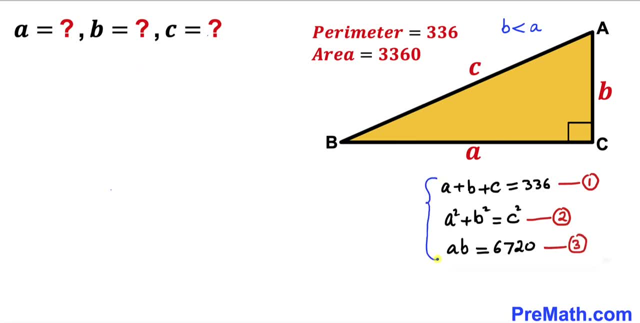 And now we can see that we got a system of these three equations And now we are going to solve for a, b and c values. And here's our next step. Let's focus on this equation one, And here I have copied it down: 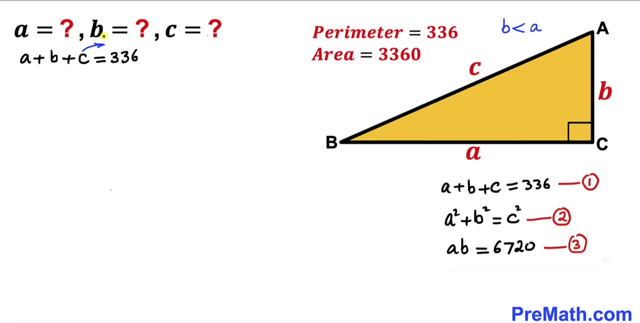 And now let me go ahead and move this c to the right hand side. Let me go ahead and take a square on both sides of these equations. And now let's recall this famous identity: a plus b- whole square could be written as a square plus b, square plus 2ab. 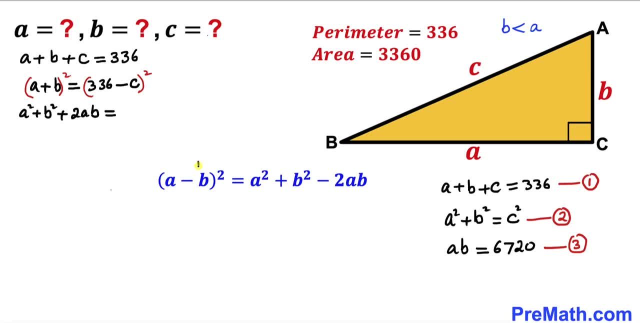 So the left hand side could be written as: And now let's recall another identity: a minus b, whole square could be written as a square plus b, square minus 2ab, And we are going to apply it on the right hand side of this equation. 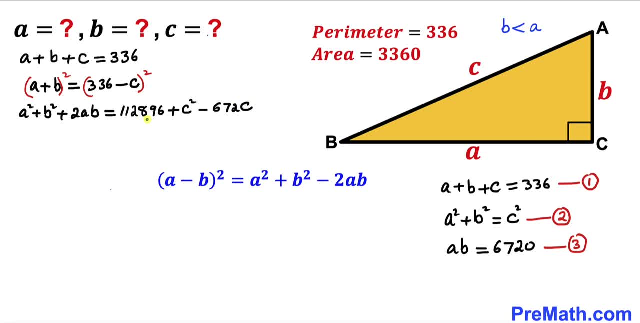 So therefore, right hand side turns out to be 112896 plus c square, minus 672 times c. And now let's make an observation. We can see that a square plus b square equal to c square from this equation 2.. So therefore I'm going to replace this a square plus b square by c square. 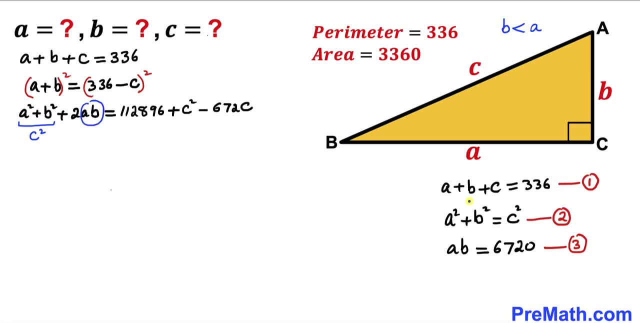 And likewise over here, a times b is equal to 6720 from this equation 3.. I'm going to replace this a times b by 6720 over here, As you can see in this next step, And here we can see that this c square and this c square, they are gone. 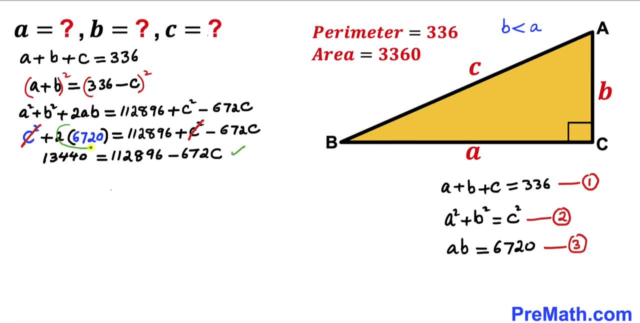 And in this Next step, 2 times 6720 gives us 13440.. And now let's go ahead and subtract 112896 from both sides, We can see this is gone, And on the left hand side, we are going to get negative 99456, equal to negative 672 times c. 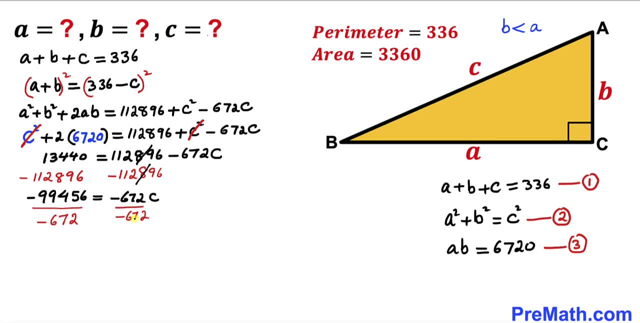 And now we are going to divide both sides by negative 672 to isolate c. We can see that this is gone. So therefore, c turns out to be equal to 148.. So that's our side length. c turns out to be 148.. 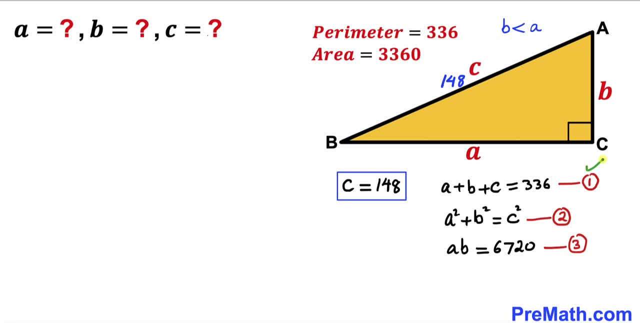 And here's our next step. Let's focus once again on this equation 1.. And here I have copied it down. And we know our c value is 148.. I'm going to substitute c over here by 148.. As you can see in this next step. 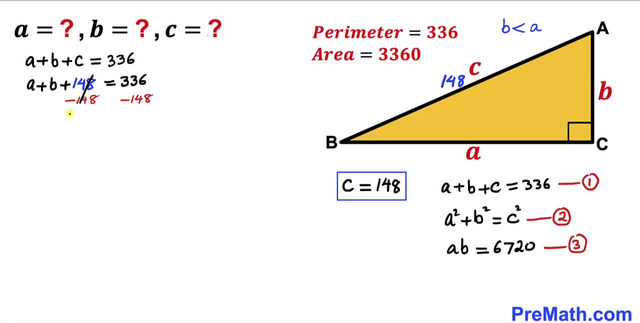 Let's go ahead and subtract 148 from both sides. This is gone. So therefore, our a plus b value turns out to be 188.. Let me call this our equation number 4.. And here's our next step. Let's focus on this equation 3.. 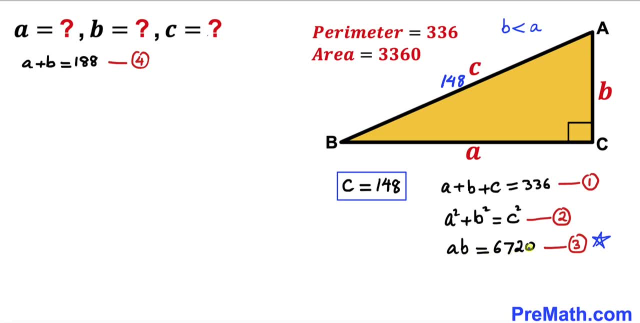 This is a times b equal to 6720.. Let me go ahead and divide both sides by a And we can see that this a and a cancels out. So therefore, our b value is going to be 6720 divided by a. 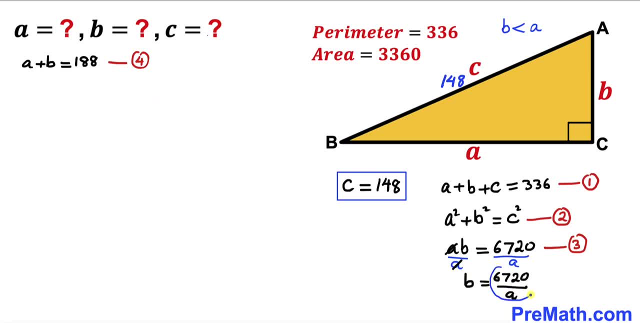 And now I'm going to substitute this b, equal to this value over here in this equation 4.. As you can see, in this next step I have replaced this b by 6720 divided by a. And now let me go ahead and multiply across the board by a to remove this fraction. 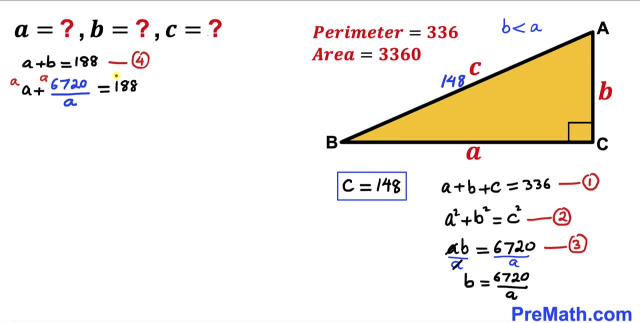 I'm going to multiply a over here, a with this second term And a on the right hand side as well, And here a times a is going to give us a square Plus this a and a cancels out. So we got 6720 equals to 1.. 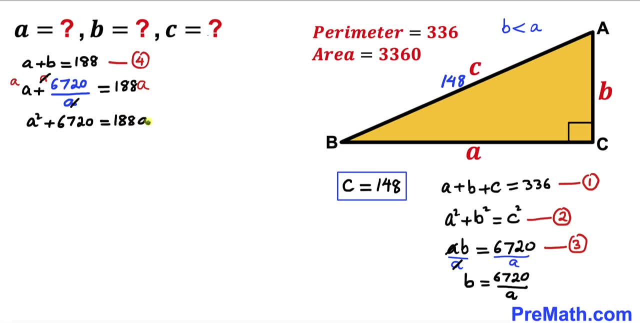 So we have 188 times a, And now let's go ahead and move this 188 times a on the left hand side, As you can see in this next step. And now we can see that we got this quadratic equation And we are going to solve it by using the quadratic formula. 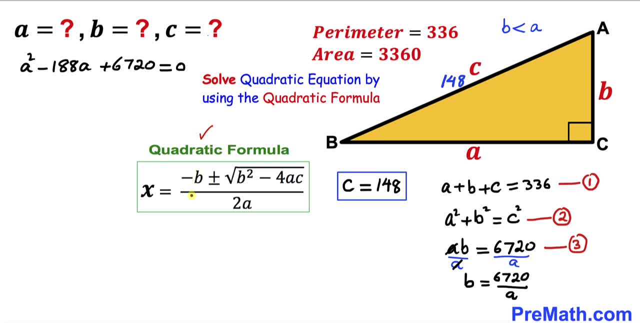 And here's our well known quadratic formula that we will be using. And let's go ahead and tweak this quadratic equation to avoid any confusion. I'm going to replace this a by Dummy variable x. Likewise this: I'm going to replace this one by dummy variable x as well. 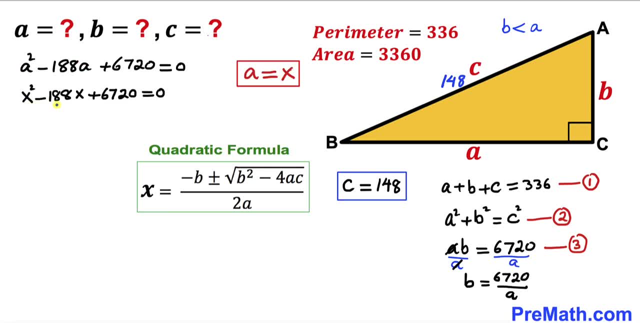 So therefore, our this quadratic equation has become x square minus 188 times x plus 6720, equal to 0.. And now we can see: our coefficient of x square is a equals to 1.. b equals to negative 188.. And our c constant is 6720.. 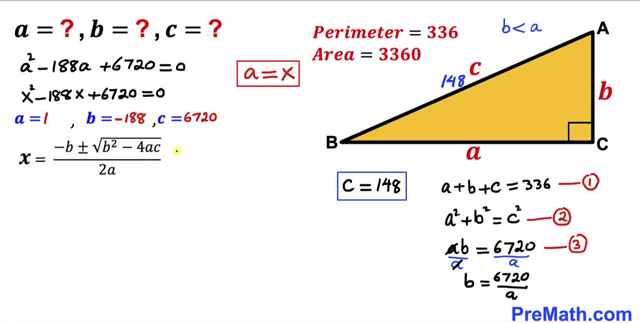 And now let's go ahead and fill in the blanks in this quadratic formula. So I can write: x equal to minus, and then b is negative 188 plus or minus. the square root of negative 188, whole square minus 4 times a, is 1.. 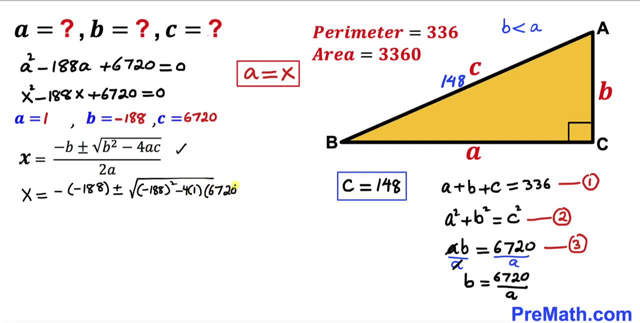 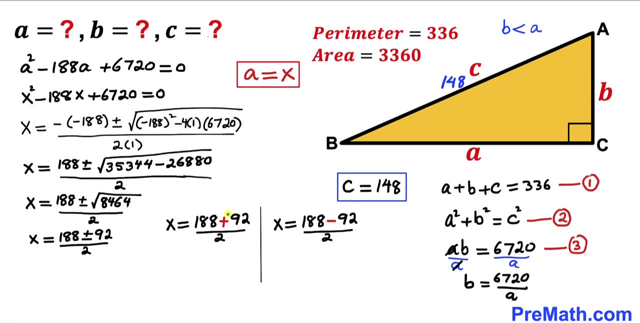 And c is 6720.. All over 2 times 1.. And here I have simplified everything. And now let's go ahead and split these two positive and negative signs. As you can see, in this next step I have put this one with the positive sign and this other with the negative sign. 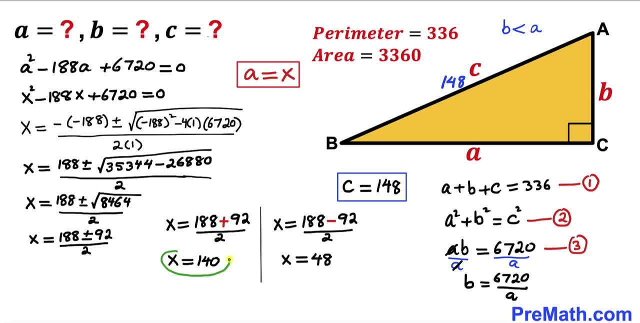 So therefore, we are ended up with two values of x: x equal to 140 and the other x value is 48. As you can see, our x value is 48. So therefore, we are ended up with two values over here, And since we put a equals to x as a dummy variable, 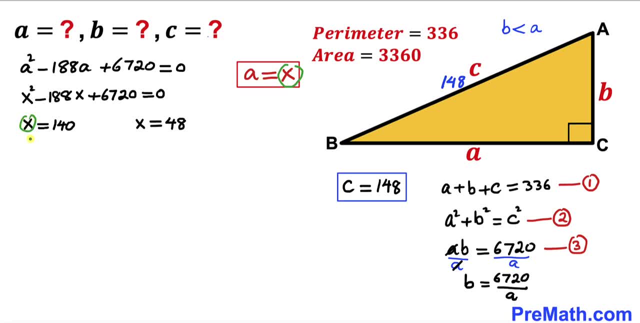 So let me go ahead and plug it back, this x as an a, And likewise x over here, a as well. So therefore we are ended up with a equals to 140 value, And the other value of a is 48.. And now let's recall the factor from the previous equations. 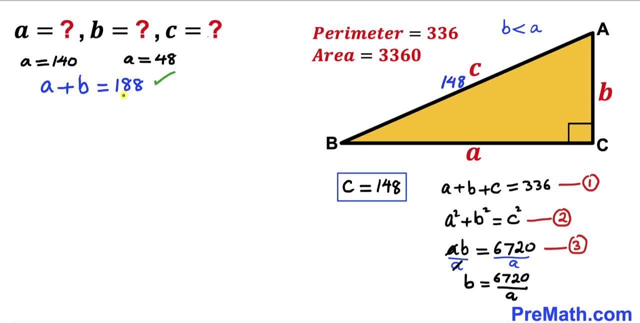 Our a plus b value equals to 180.. And now let's go ahead and substitute this: a equals to 140 value in this equation. So therefore we got 140 plus b equals to 188.. So let's go ahead and subtract 140 from both sides.